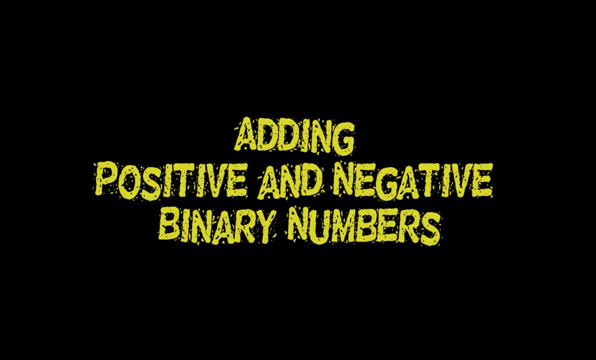 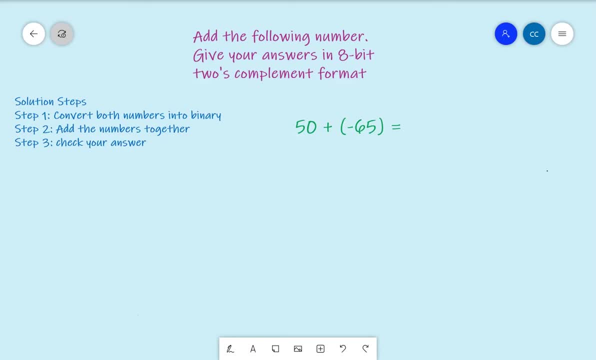 This question is asking you to add the numbers 50 and negative 65 together and express your answer in 8-bit 2's complement. I've written down a couple of steps here for the solution, just to help you with that. So convert both numbers into their binary equivalent. That's the first thing. 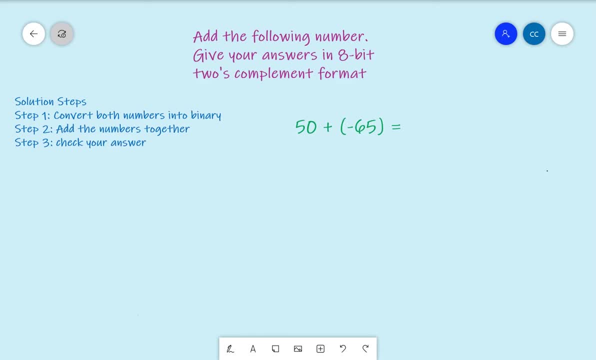 you want to do, Then add the numbers together and then check your answer. So we've got two numbers here. We've got 50,, which is a positive number, and we've got negative 65,, which is a negative number, And, as you know, all negative numbers are expressed in 2's complement in a. 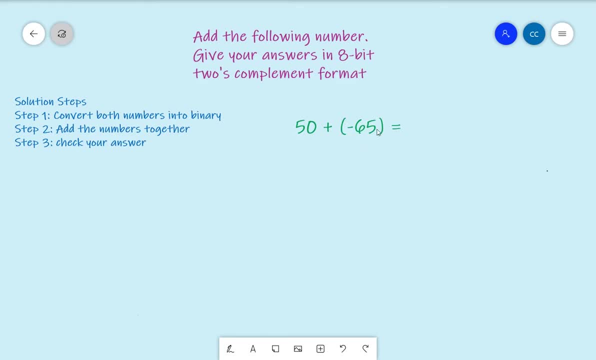 computer system. So negative: 65 is 2's complement, 50 is not 2's complement, So let's start with the first number, 50.. Let's put the place values in, So 1,, 2,, 4,, 8,, 16,, 32,, 64 and 128. 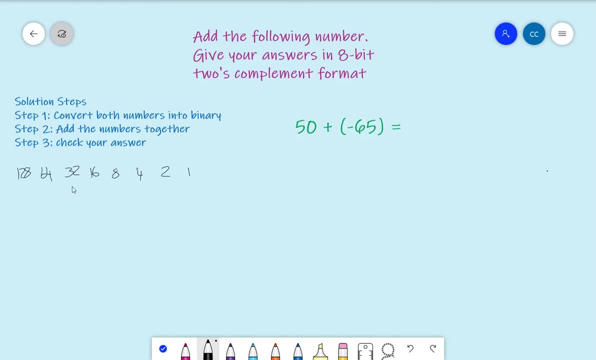 We know that 50 is made up of 32.. We've got 18 left, so we need a 16 and a 2.. So we don't need those, So we'll put zeros in there. So 50 is 00110010.. Negative 65 needs to be converted. 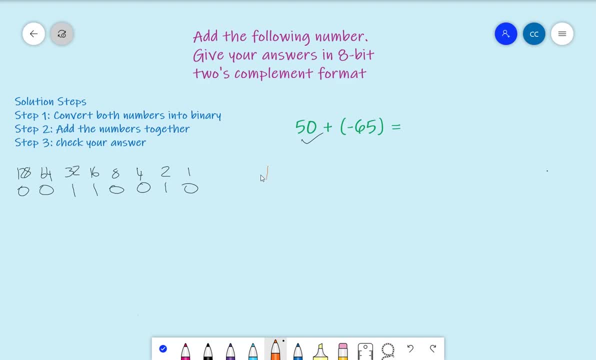 using 2's complement. So let's put down 2's complement and remember how to do this. So 2's complement. There are three steps. So step one: what is it? Find the positive. Step two: can you remember what that is? That's flip. And step three: can you? 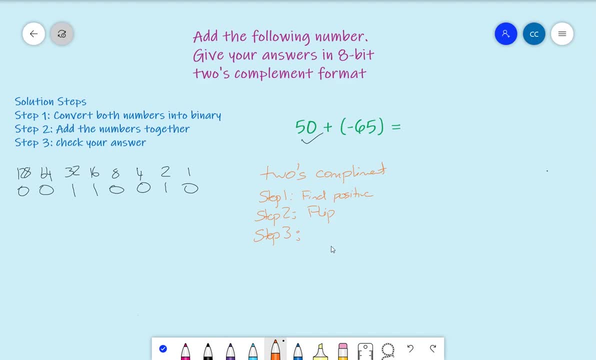 remember what that is. Add one. Okay, let's do that. So put down our grid as normal. So we've got 1, 2,, 4, 8,, 16,, 32,, 64 and 128.. So the first thing we're doing is finding the positive 65.. 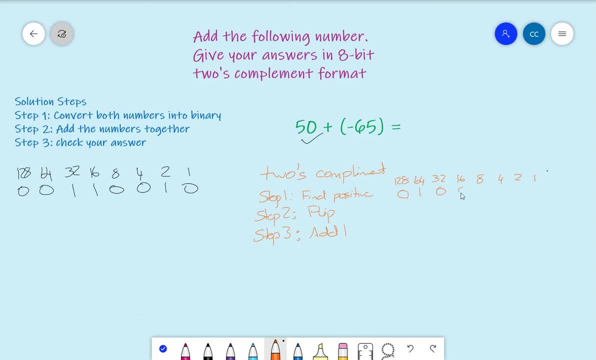 So we don't need that. we need a 64 and we also need a 1.. 64 and 1 is 65.. Now we need to flip, so 1 0, 1, 1, 1, 1, 1, 0.. 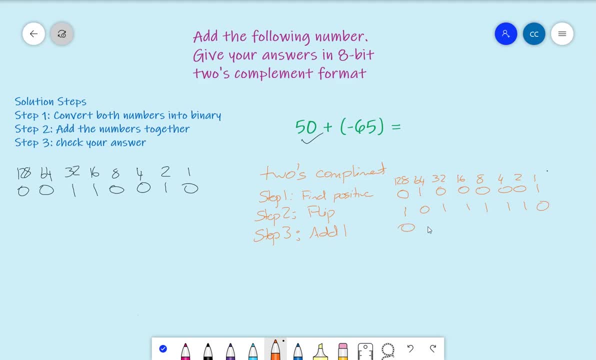 And now we need to add one. So let's put in a 1. And I like to put a line above and below it, just so that I'm clear on what it is that I'm adding. 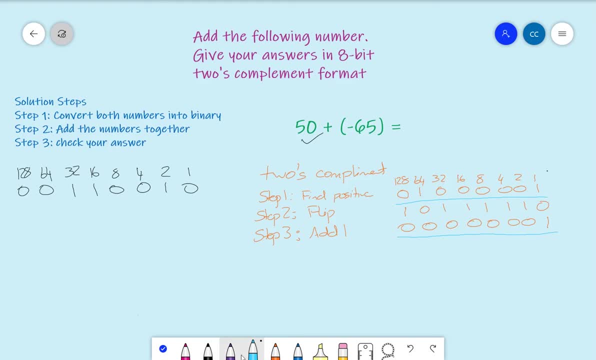 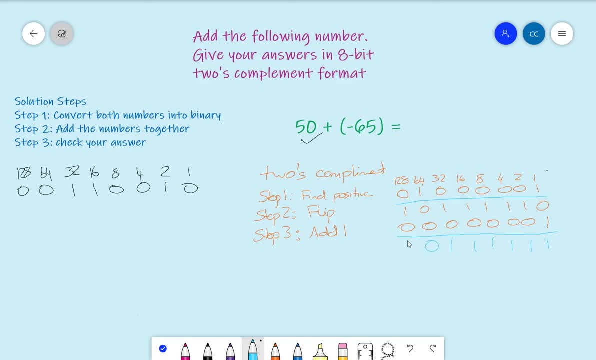 1 plus 0 is 1.. 0 plus 0 is 0.. 1 plus 0 is 1.. So there is the answer. This is minus 65.. Now we can test this to make sure it is minus 65 before we go any further. 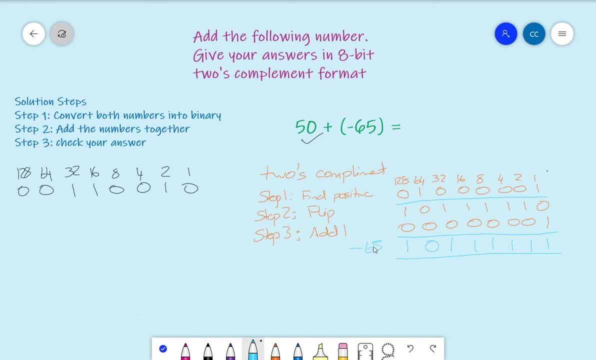 So let's write down here: minus 65.. And we know how to test 2's complement, don't we? This most significant bit, which in this case is the 2 to the power 7, is minus 128.. Plus 32,, plus 16,, plus 8, plus 4,, plus 2, plus 1.. 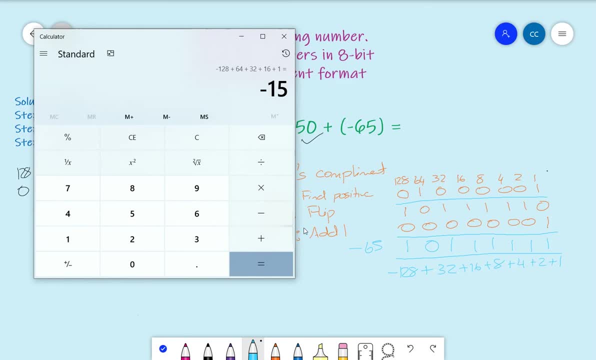 So let's get our calculator and check that. So we start with 128, change the sign to negative, plus 32,, plus 16,, plus 8,, plus 4,, plus 2, plus 1, and that's minus 65.. 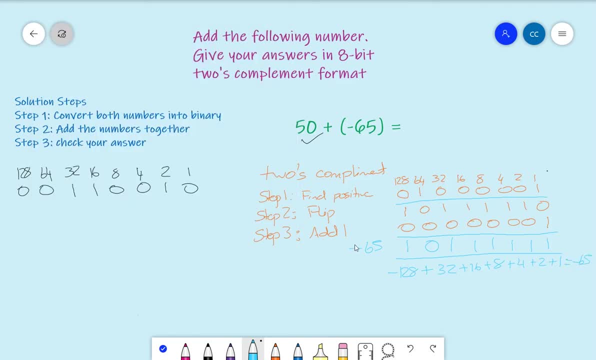 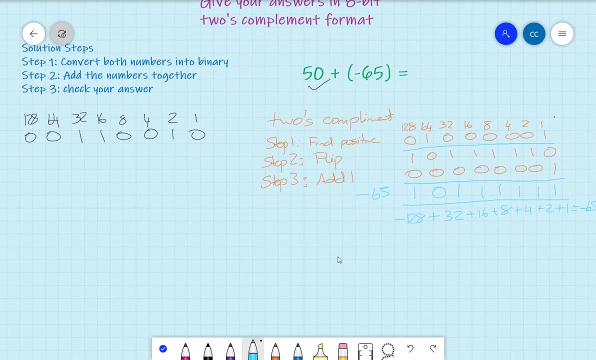 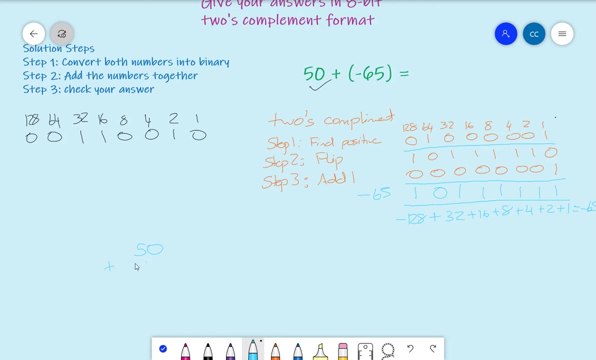 So that equals minus 65.. With confidence we can add these two binary conversions together. So let's do that now. So we'll start off with 50.. We'll just write 50 over there And then we'll write plus minus 65.. 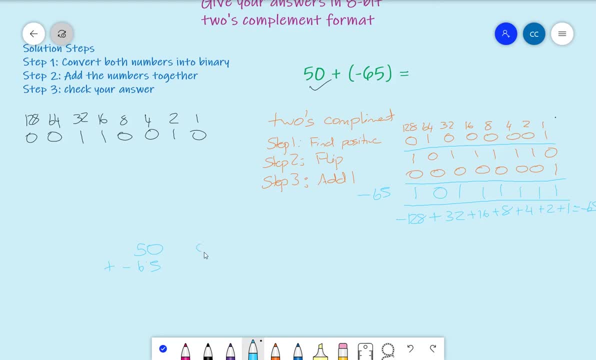 And then we'll write down what they are. So we know that 50 is 0.. So we know that 50 is 0.. So we know that 50 is 0, 0, 1, 1, 0,, 0,, 1, 0.. 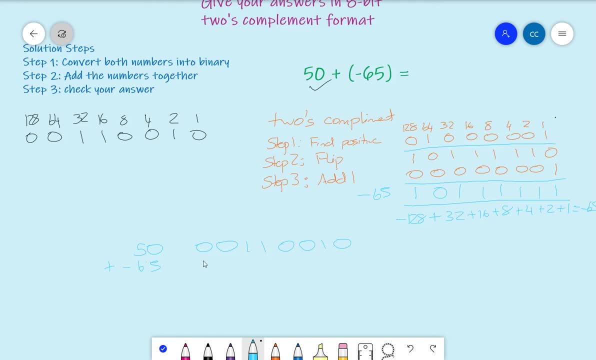 And we know that minus 65 is 1, 0,, 1, 1,, 1,, 1,, 1,, 1.. Right, let's write these together. So 0 plus 1 is 1.. 1 plus 1 is 2.. 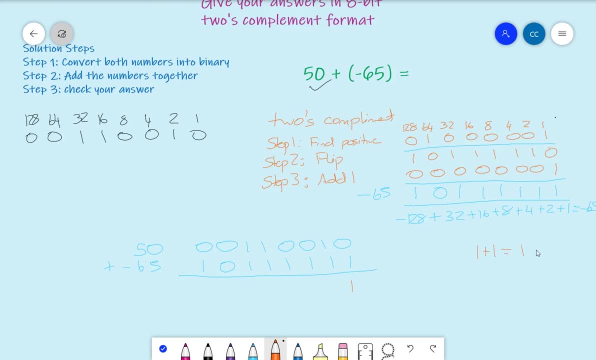 Let's write that down: 1 plus 1.. 1 plus 1 is 2.. Yeah, So we write down 2.. And we carry the 1.. 1 plus 0 plus 1 is 2.. Put down the 0,, carry the 1.. 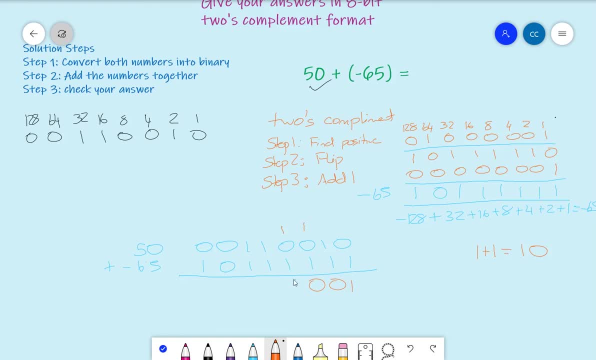 1 plus 0 plus 1 is 2.. Put down the 0, carry the 1.. Put down the 0, carry the 1.. So 1 plus 1 plus 1.. Let's do that one. 1 plus 1 plus 1 is 3.. 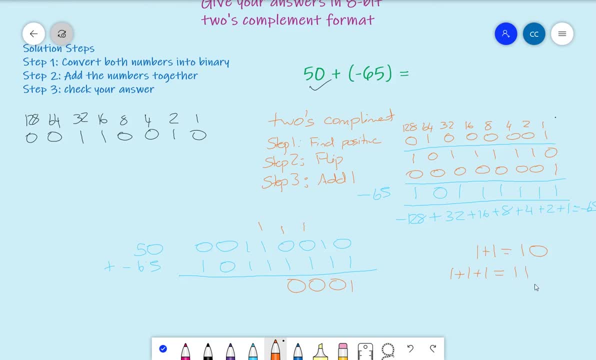 1 plus 1 plus 1 is 3.. A 1 and a 2. Together gives you 3.. So we put down a 1 and carry the 1.. 1 plus 1 plus 1 is 3.. 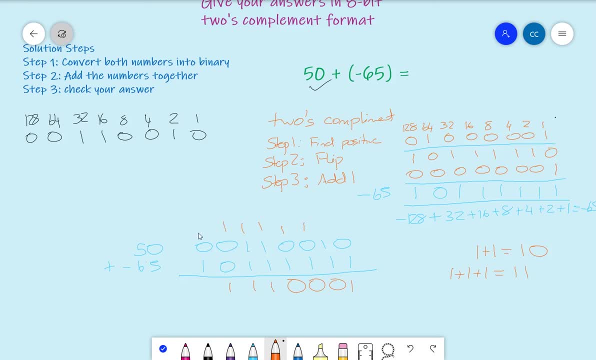 Put down the 1, carry the 1.. 1 plus 0 plus 0 is 1.. 0 plus 1 is 1.. So this is our answer. The answer is in 2's complement, But we need to check it to make sure it is correct. 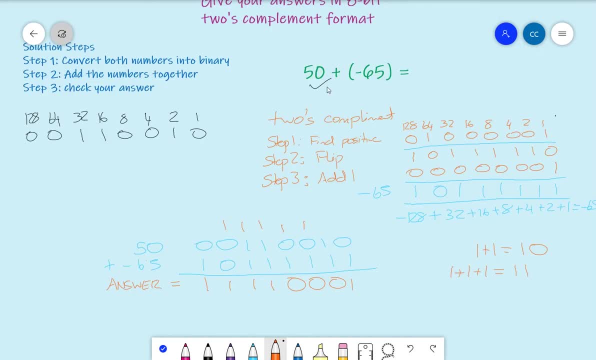 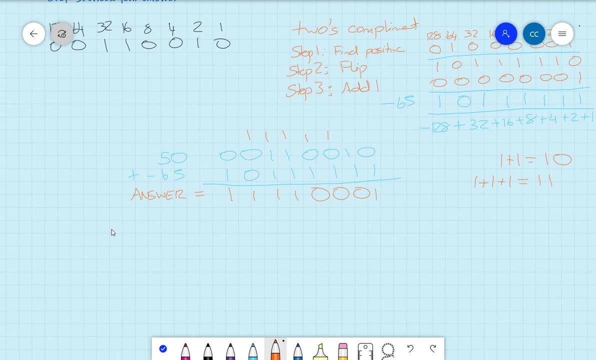 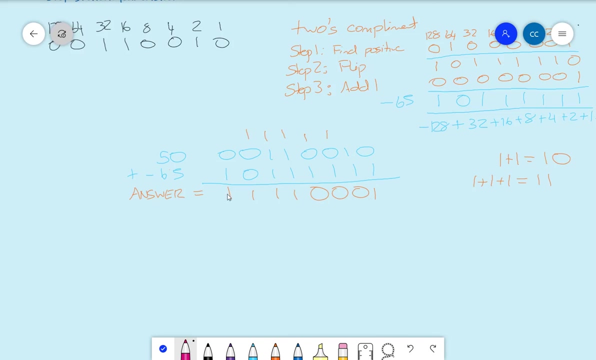 So we know just in our heads that 50 plus minus 65 is minus 15,, don't we? So let's go ahead and check this to see that we are correct. So it is in 8 bits, So this most significant bit is negative: 128 plus 64 plus 32 plus 16 plus 1..